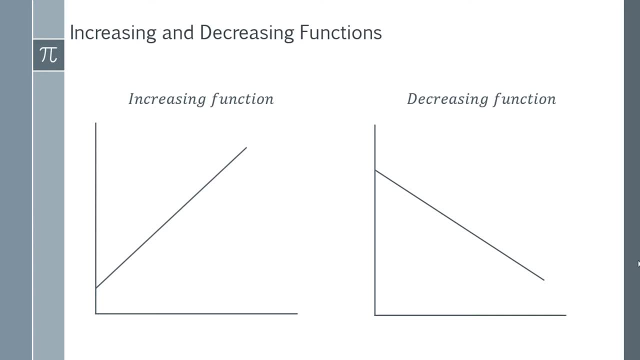 actually state a criteria mathematically that shows you whether a function is increasing or decreasing, And the rule is that if the derivative f dash of x is greater than zero- so a positive number- you have an increasing function, Whereas if f? dash of x is less than zero, that means that 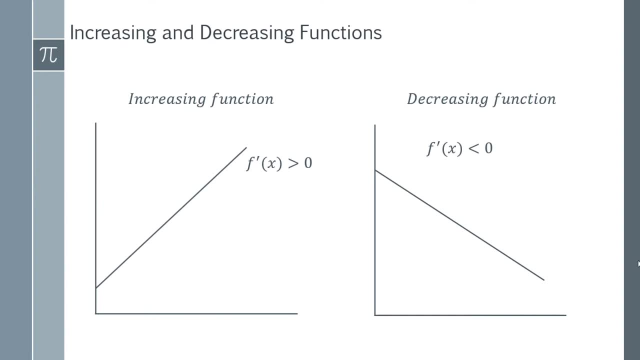 you have a decreasing function, And if a question asks you to show that a function is always increasing or always decreasing, you have to attach another criteria to this, which is that these rules have to apply for all values of x. You may have a function that is increasing and then 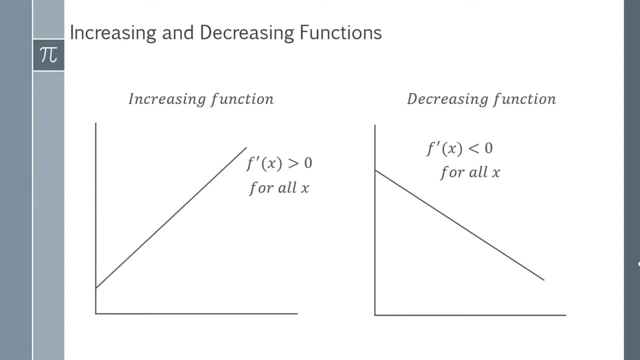 decreasing and then say increasing again. In that case you would have: between certain values you would have f dash of x is greater than zero, so it's increasing. And for other values you would have f dash of x is less than zero, So that function wouldn't always be increasing. or 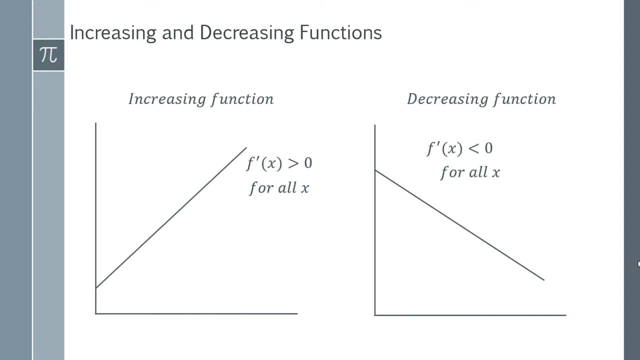 decreasing, But you can actually find the hypothesis so awesome. Thanks for looking. See you in a few years, See you soon. Bye. father out its behavior between each point by applying these rules, And so these rules work for any problem and are universal for increasing and decreasing functions. So let's look at two work. 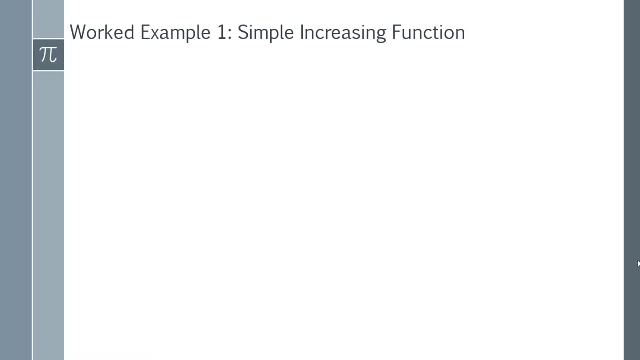 examples. So for our first work example, we're going to look at a simple increasing function, And so the question asks: show that this f of x is an increasing function. So what we need to do is prove that for every single value of x, the function is increasing. So the first step is: 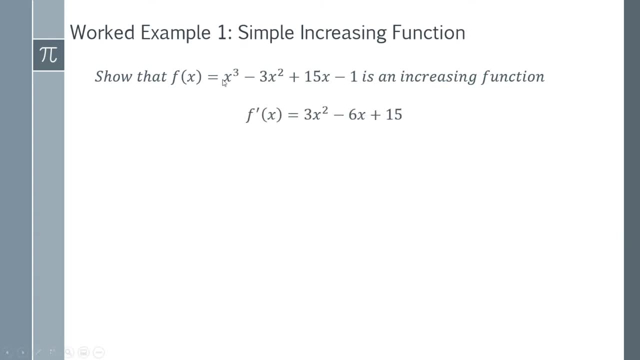 to simply find the derivative, And that's very straightforward. The 3 comes to the front subtract 1. We get the 3x squared term. Then this 3 is multiplied by the 2. That gives us the minus 6x. And then we drop the x here, leaving plus 15.. And the derivative of this is obviously 0.. 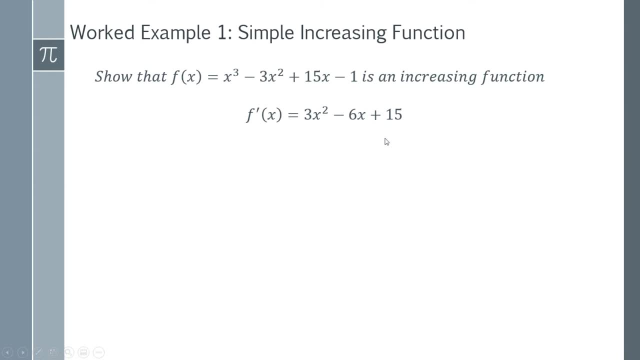 So we get our f dash of x. What we need to do is find some way to show that, for every single value of x, that this is going to be greater than 0.. And because this is a nice, simple one, one technique you can use is to complete the square. 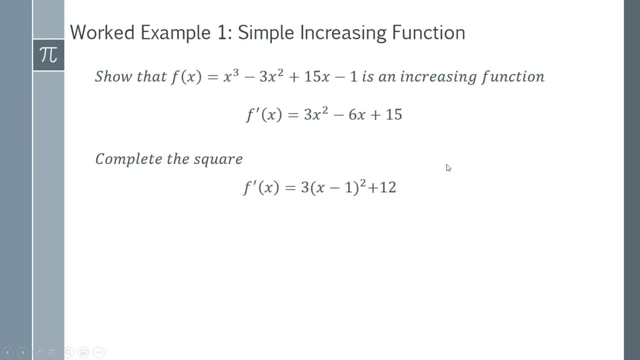 So we're going to complete the square here, And so we end up with this expression. when we complete the square, You'll notice there's a factor of 3 that can come out of these, And then, when you do that, you're going to end up with a 2, which you have, And then that goes in there, And then you 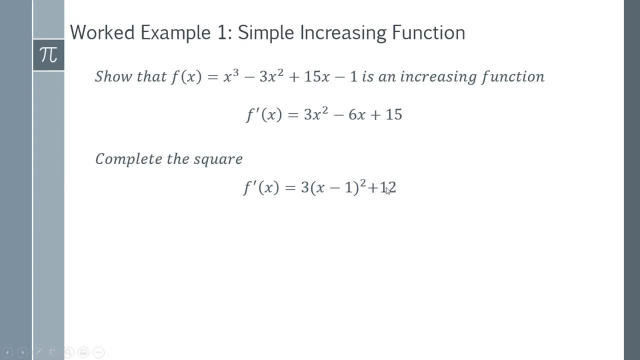 want to make sure that plus 15 is there, And then you want to make sure that plus 15 is there, And the way that you can do that is by having a plus 12 on the end. So we've now completed the square. 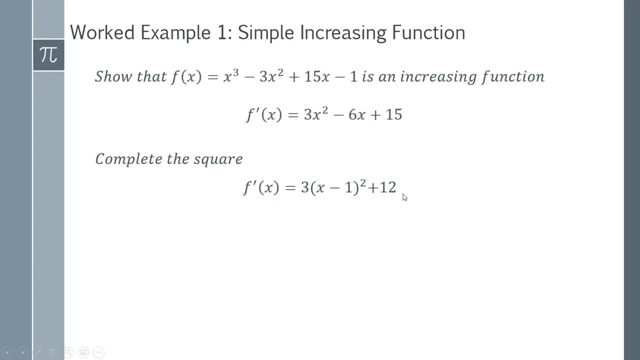 And we've got a nice expression, And when you look at this, it's very easy to work out what the absolute lowest possible value of f dash of x is. And so if we imagine that x equals 1, that will make this whole bit be 0. And so the lowest possible value that you could ever get. 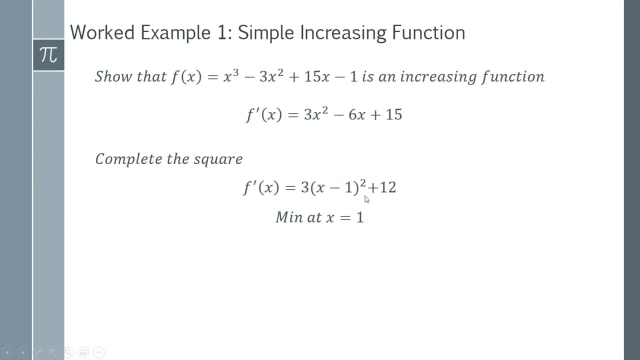 remember, this is squared, So any negatives are going to become positive. So the lowest possible value that you could ever obtain for the derivative is going to be 12.. And that occurs when all of this becomes 0.. So we've shown that the lowest possible value that you could ever obtain for the derivative is: 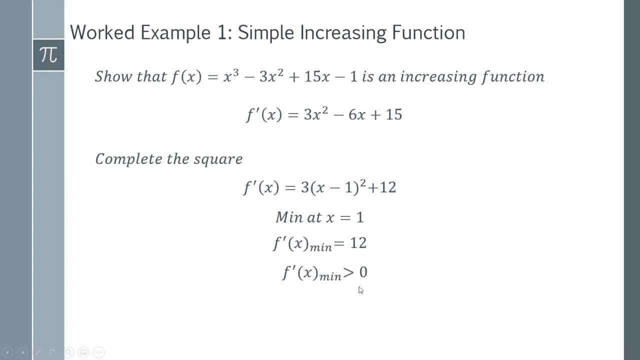 12. That is, of course, greater than 0. So the lowest possible value is greater than 0. So every other value is going to be greater than 12. So every other value is going to be greater. 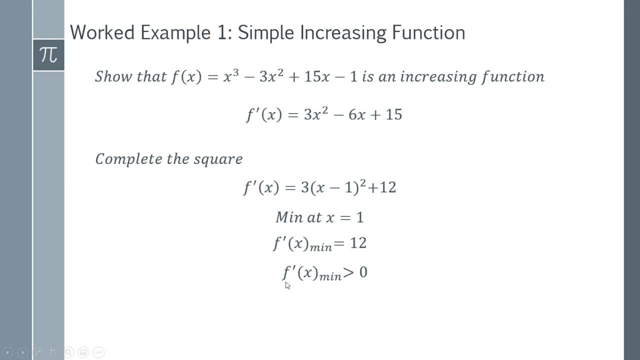 than 0. So therefore, for every single value of x, the function is going to be an increasing function. So we can conclude that this is an increasing function. So, basically, what we've done is found the derivative and then found some way to prove that every single possible value is going to be. 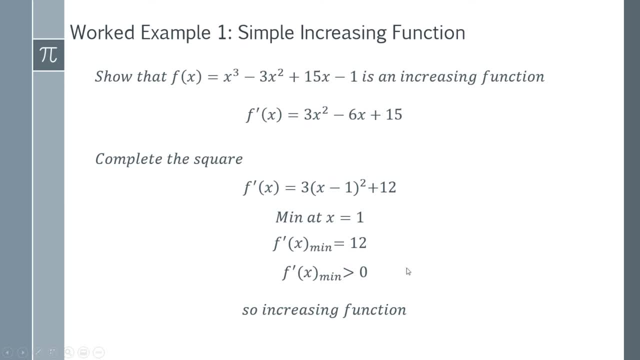 positive, And so it's therefore satisfied our condition for an increasing function. Let's look at a second work example to prove that a function is a decreasing function, And so the question is: is it a decreasing function, function? And so the question is: show that f of x equals. this is a decreasing function. So we've. 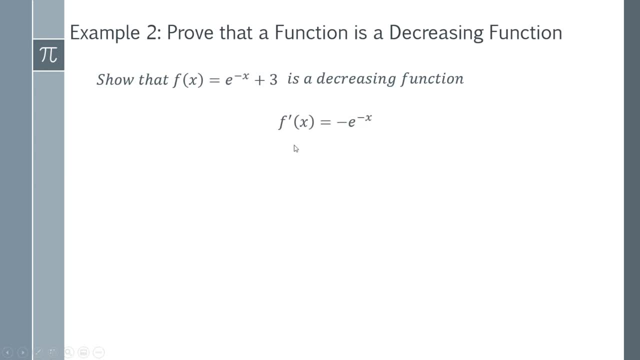 got something a little bit more complicated. As always, the key is to start by finding the derivative, And of course the derivative of e to the x is e to the x, So e to the minus x. we end up with a minus here and then we get this expression. Now this one can be solved by just 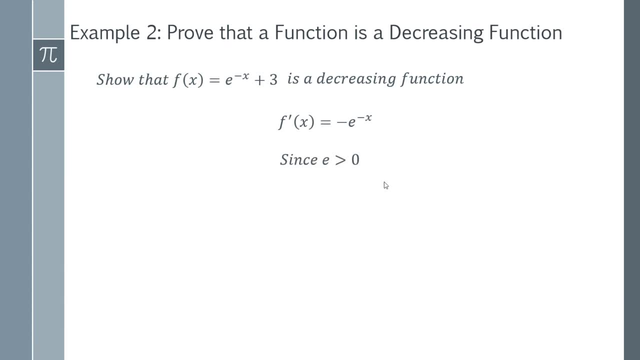 thinking about the e to the x function, And so we know that e is a positive number, e is two point something, So it's just a number, it's a constant that is greater than zero, And basically any number to the power x is going to be greater than zero. you can try that with lots of negative.